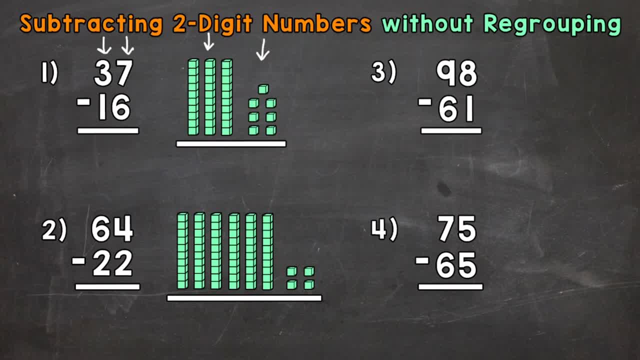 seven ones. Now that we have that, we can subtract, And when we subtract whole numbers we start with the ones place. So we have seven ones minus six ones. So let's subtract or take away six ones: One, two, three, four, five, six. 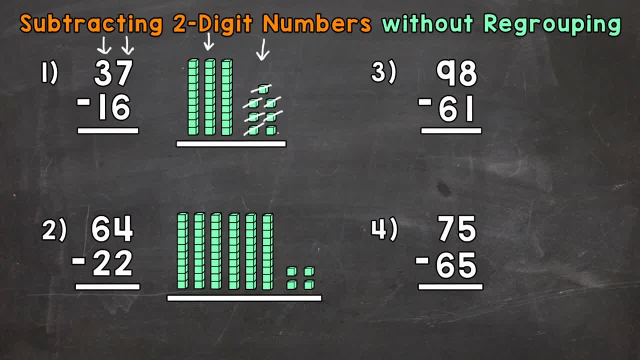 Now we need to see how many we have left. Well, one, So we put a one in the ones place in our answer. Now we move to the tens. So we have three tens minus one ten. So let's subtract or take away one ten One. Let's see how many we have left One. two, So we put a two in the tens place in our 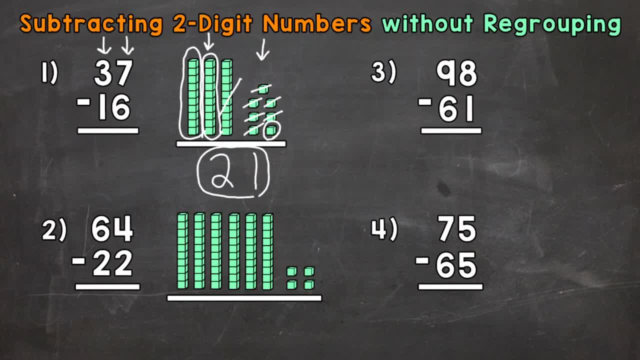 answer, Our final answer 21.. Let's go over to the left, to the original problem, and solve it over there as well and see if we still get 21.. Start with the ones: Seven minus six gives us one. Now for the tens: Three tens minus one, ten. That gives us two tens in our answer for a final answer of 21.. 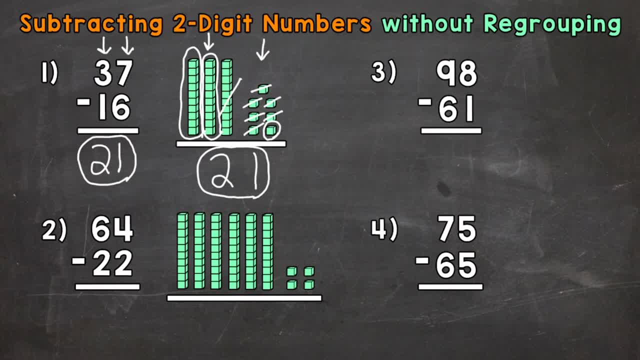 Let's move on to number two, where we have 64 minus 22.. So, starting with 64 and subtracting or taking away 22.. 64 is represented by base, 10 blocks, Six 10s and four 1s. Let's start by subtracting the 1s, So 4 minus 2.. Four 1s. 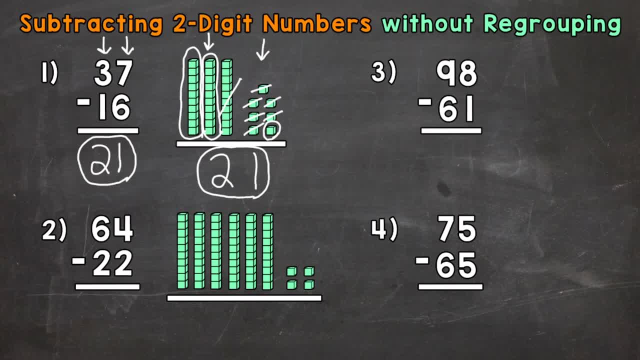 and we are subtracting or taking away two 1s. Let's subtract those two 1s. One two. Let's see how many. we have left One, two. So we put a two in our answer in the ones place. Now we move to. 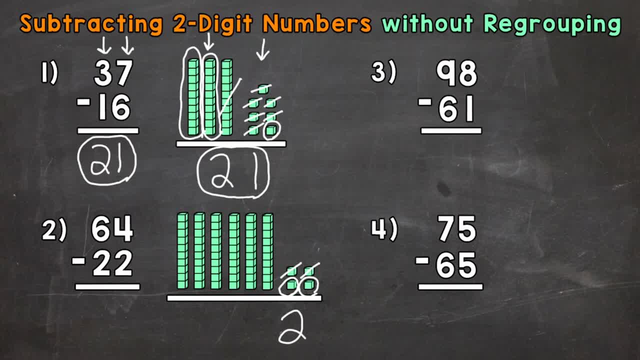 the 10s. So we have six 10s minus two 10s. So let's subtract those two 10s from the six, One, two. Now we need to see how many we have left. So one, two.